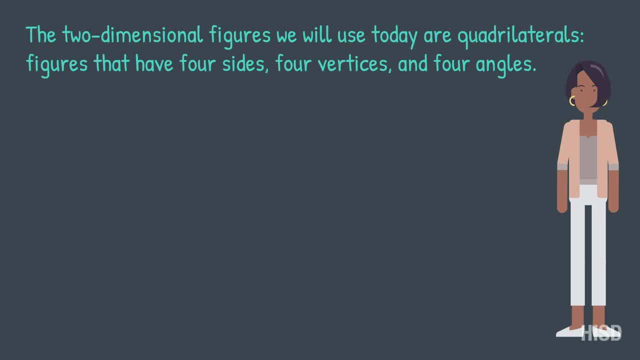 The two-dimensional figures we will use today are quadrilaterals, figures that have four sides, four vertices and four angles: Square, rhombus, isosceles, trapezoid, rectangle, parallelogram, right trapezoid. 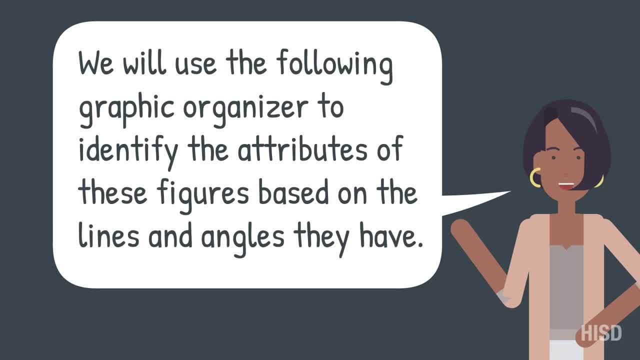 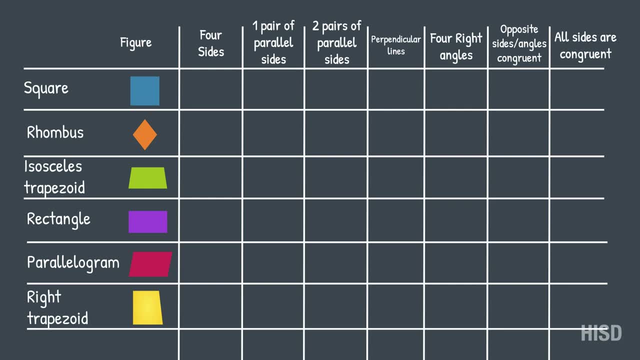 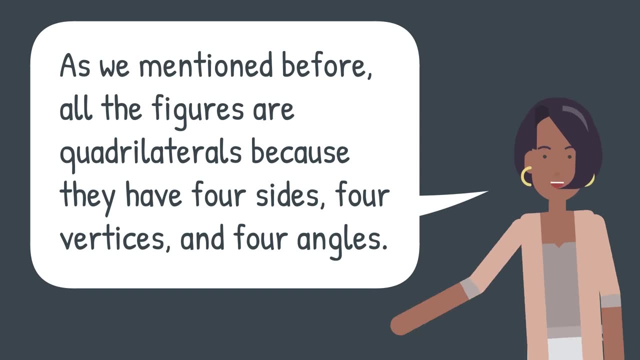 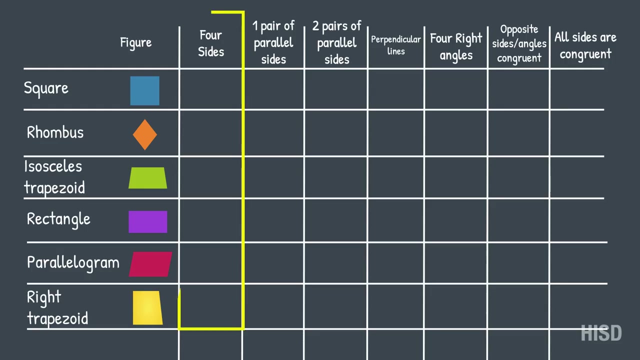 We will use the following graphic organizer to identify the attributes of these figures based on the lines and angles they have. As we mentioned before, all the figures are quadrilaterals because they have four sides, four vertices and four angles. We will check the column four sides for all these figures. 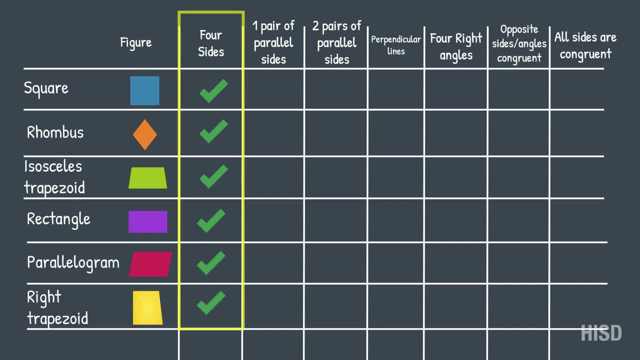 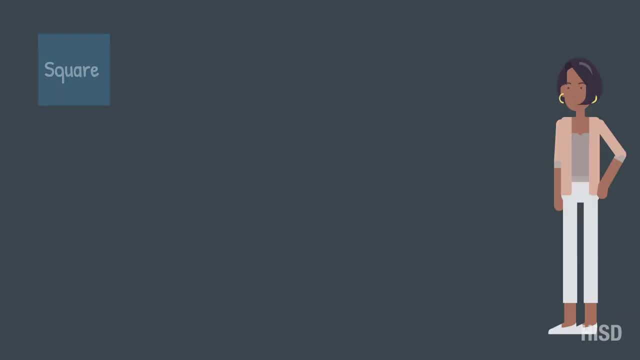 We will use the following graphic organizer to identify the attributes of these figures based on the lines and angles they have. Now we will count the number of parallel sides. each figure has: Square: one pair of parallel sides. two pair of parallel sides. Rhombus: one pair of parallel sides. two pair of parallel sides. 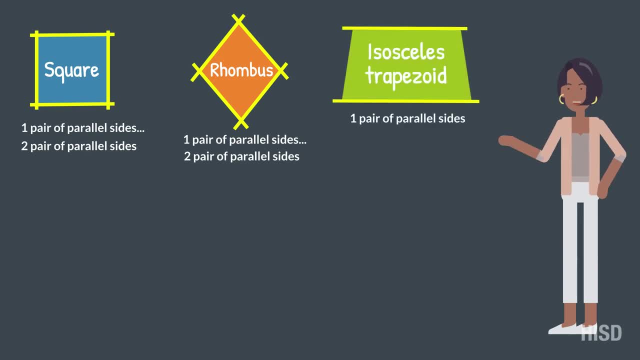 Isosceles: trapezoid: one pair of parallel sides. Rectangle: one pair of parallel sides. Page number three: What is it? Let me think I forget the sign name. sides: two pair of parallel sides. Parallelogram: one pair of parallel sides. 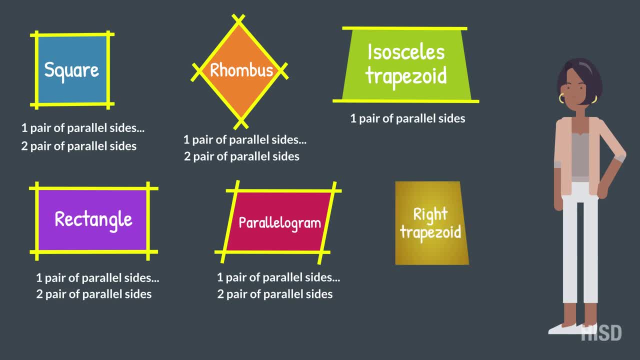 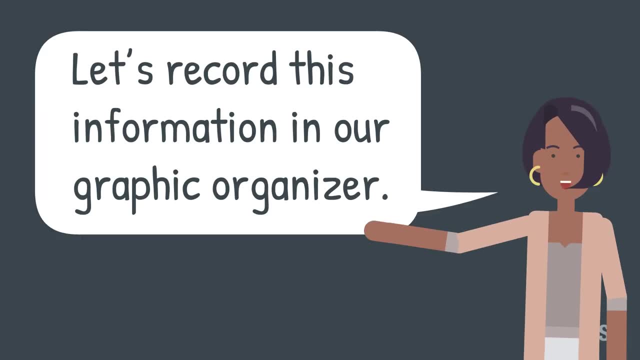 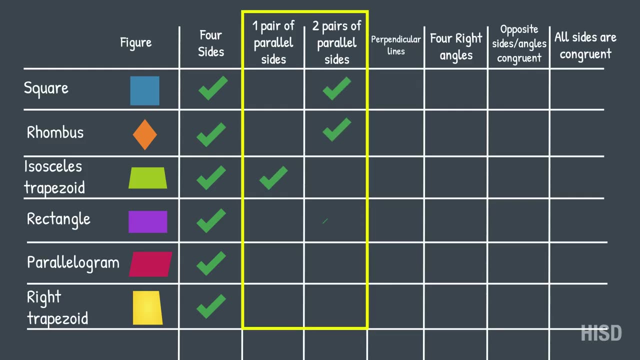 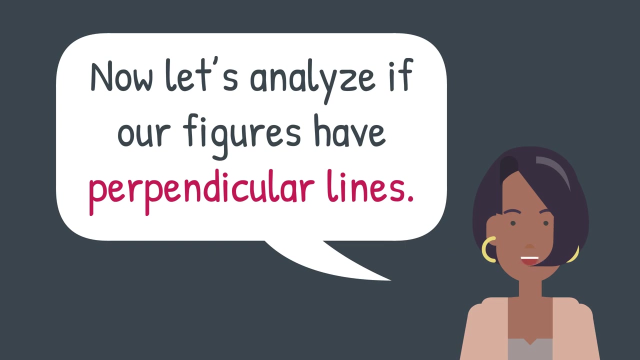 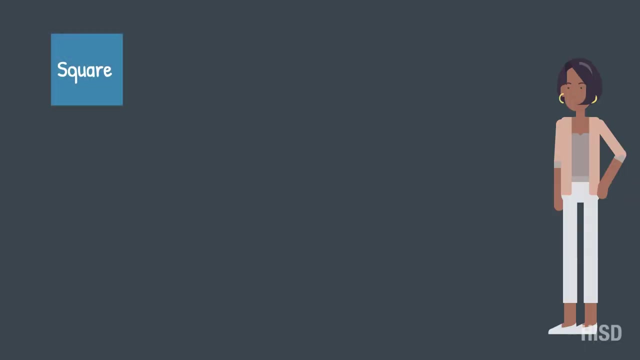 two pair of parallel sides. Right trapezoid: one pair of parallel sides. Let's record this information in our graphic organizer. Now let's analyze if our figures have perpendicular lines. Perpendicular lines will form right angles when they intersect Square, all the sides when they intersect form. 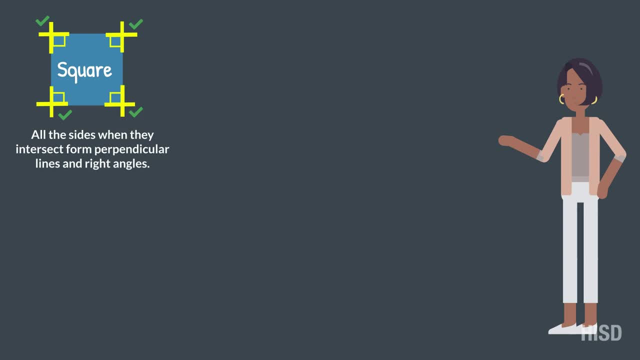 perpendicular lines and right angles. Rhombus: it does not have perpendicular lines nor right angles. A sausalese trapezoid: it does not have perpendicular lines nor right angles. Rectangle: all the sides when they intersect, form perpendicular lines and 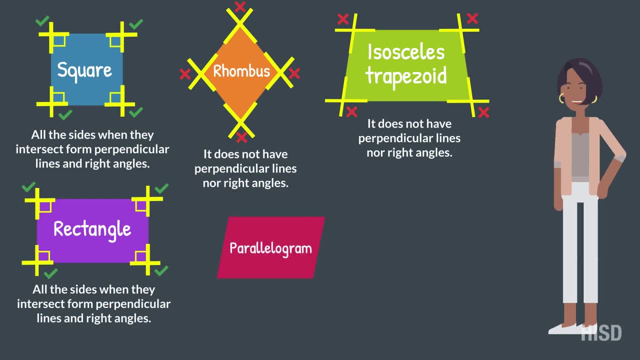 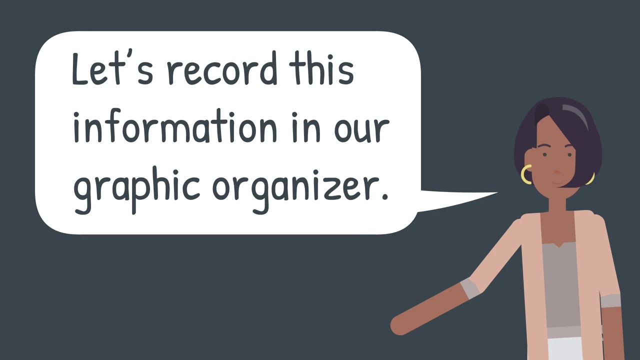 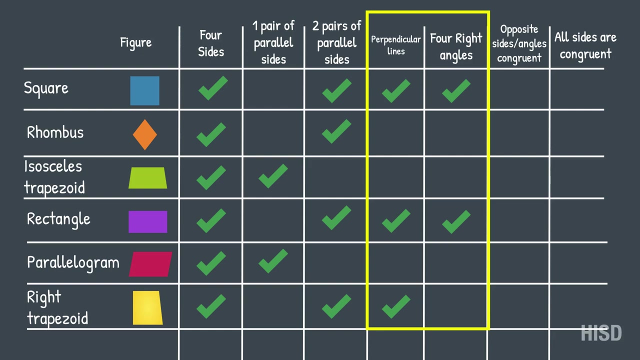 right angles- Parallelogram. it does not have perpendicular lines, nor right angles. Right trapezoid. this figure does have some perpendicular lines, but not all the lines are perpendicular. Let's record this information in our graphic organizer. Now let's analyze if the opposite sides and angles of the figures are congruent. 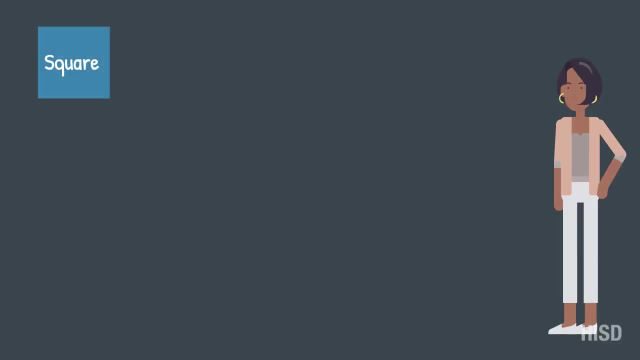 or have the same size Square. top and bottom sides are congruent and left and right sides are congruent. We can see that all the sides are the same size. therefore, all sides are congruent. Rhombus: opposite sides are congruent and all the sides are the 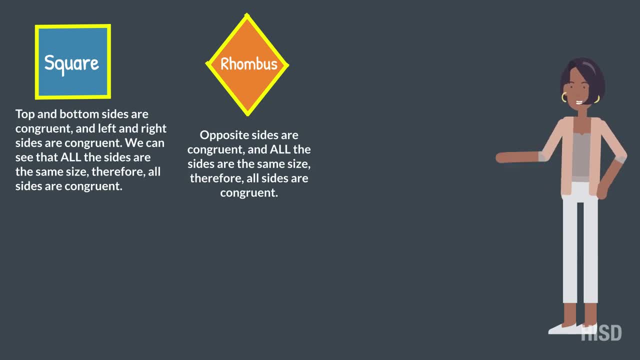 same size. therefore, all sides are congruent. measures: trapezoid: top and bottom sides are not congruent, Only the left and right sides are congruent. Rectangle: Top and bottom sides are congruent and left and right sides are congruent. 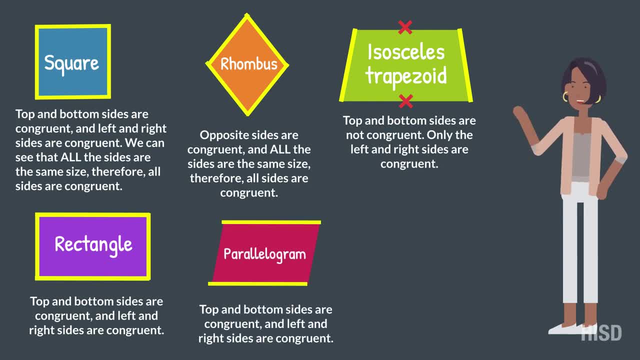 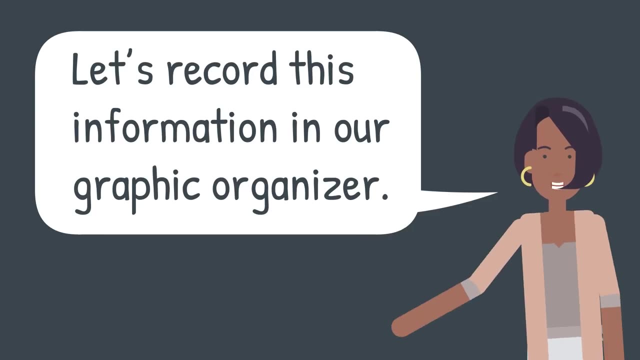 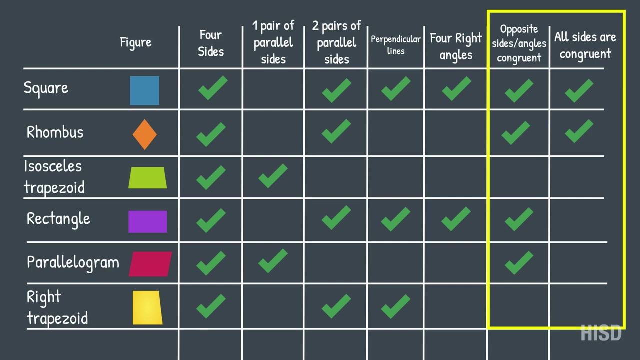 Top and bottom sides are congruent and left and right sides are congruent. Write trapezoid: None of the sides are congruent. Let's record this information in our graphic organizer. Using the graphic organizer that we created, we can classify the two. 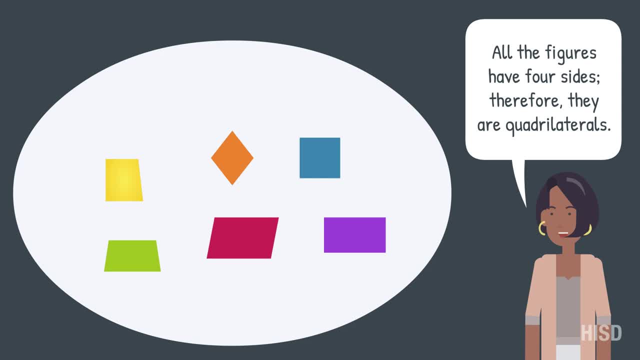 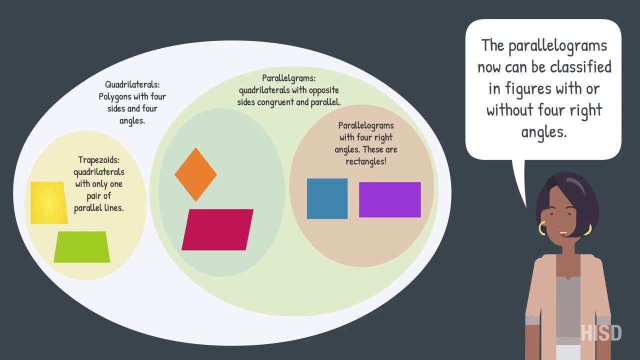 dimensional figures as follows. All the figures have four sides, therefore they are quadrilaterals. Then we can see that some figures have only one pair of parallel lines and others have two pairs of parallel and congruent lines. The parallelograms now can be classified in figures with or without four right. 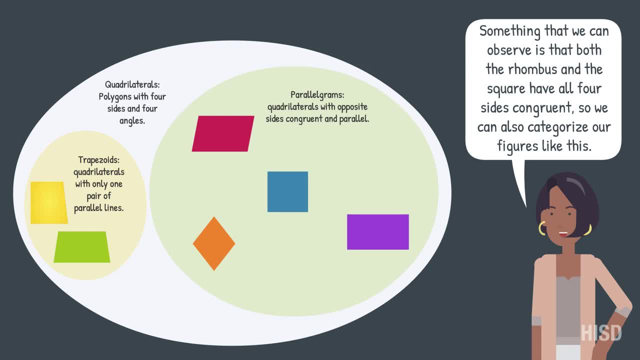 angles. Something that we can observe is that both parallelograms can be classified in figures, with or without four right angles. Something that we can observe is that both- Both the rhombus and the square- have all four sides congruent, so we can also categorize.